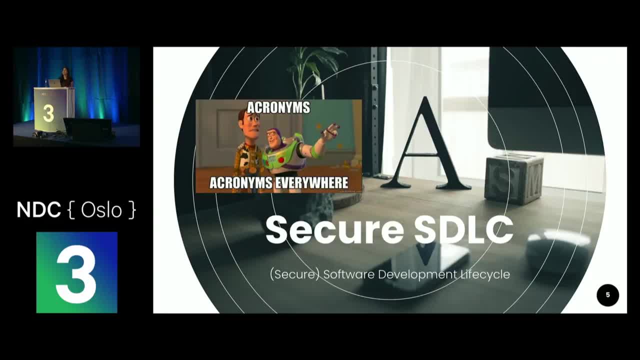 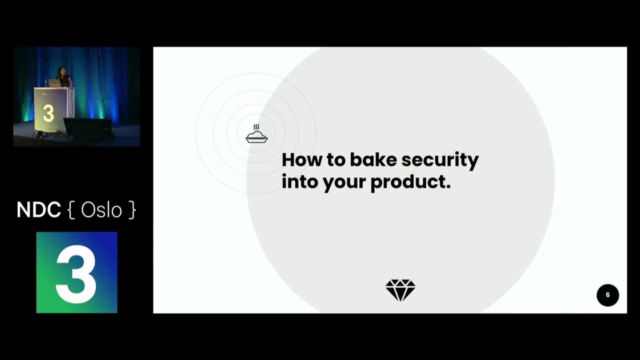 it just secure SDLC Or secure SDL, or I believe Microsoft is Microsoft SDL. So it's all essentially the same thing. They just name different steps by different actual names. Okay, so it's basically just baking security into your product. It all means the same thing And it's a multifaceted 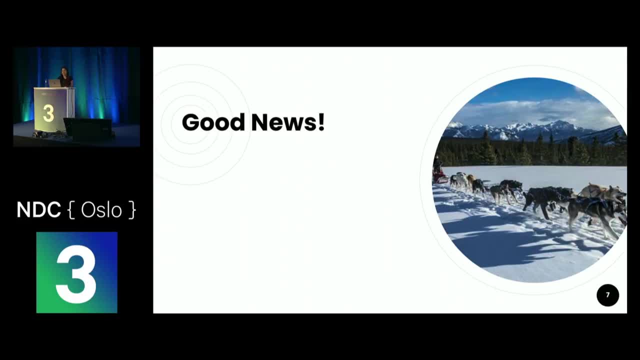 approach. hence the diamond. But good news is that it is, it's a partnership, And it's not entirely on you. It's not entirely on you. It's not entirely on one person. in general, It really takes a team. So in this picture, 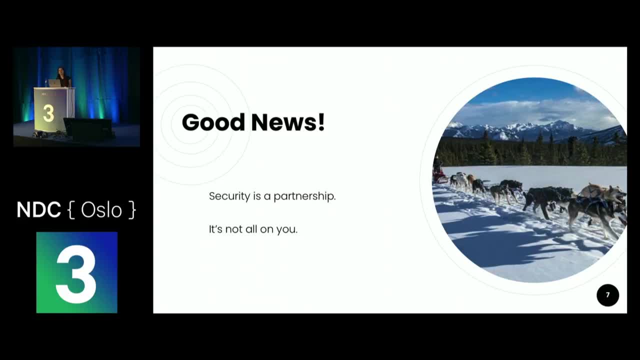 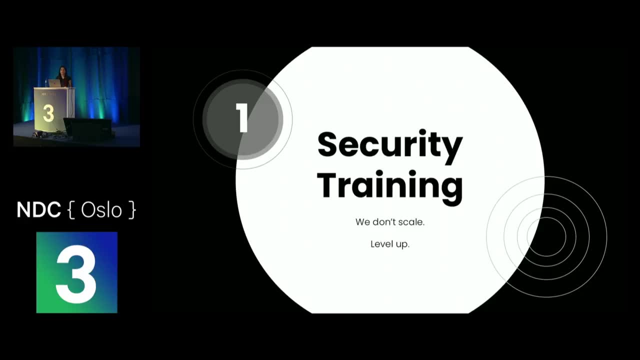 all the dogs there are us as a team and we're pulling the product across the line. So that basically leads to the first step, which is security training. So security training is really important because the amount of security engineers to everyone else in the 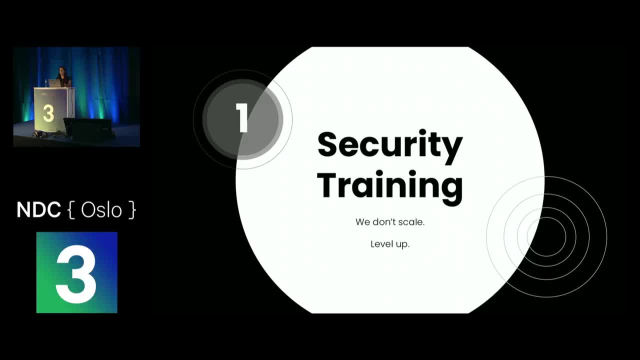 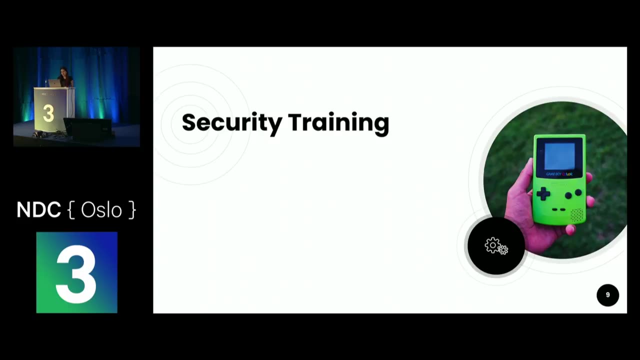 company is so far from one to one that we can't see what's going on all the time. And it's really difficult to be able to bake security in when you have a smaller team, Not that great of ratios. So the solution is to level up, level everyone else up. So 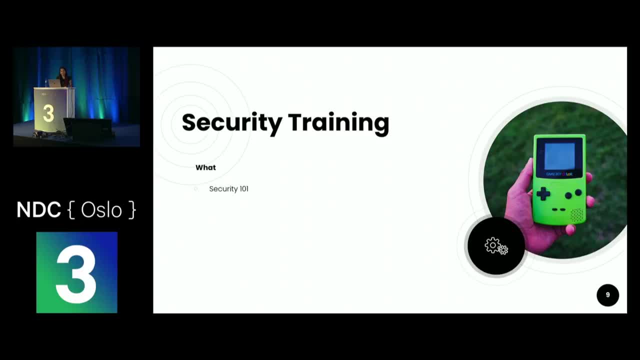 security training. What it is is security 101.. It's basically going over some of the common issues so that you know generally what to look for, so you don't fall for things, Some indicators kind of like red sirens. When you see it you're like, okay, I should. 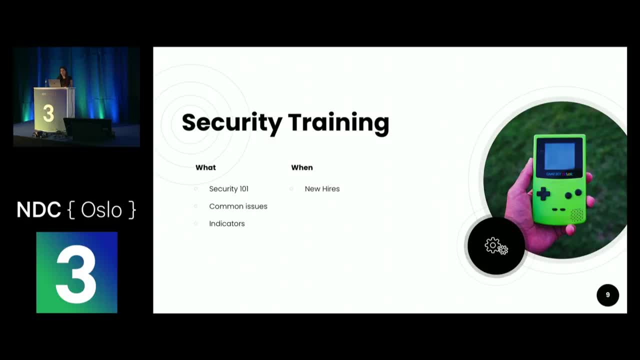 probably check that out And when you would do it. so I specifically do it with all new hires. Okay, So when you hire engineers, they have this fresh outlook and they want to know what's important to the company And as security is something that's extremely important to. 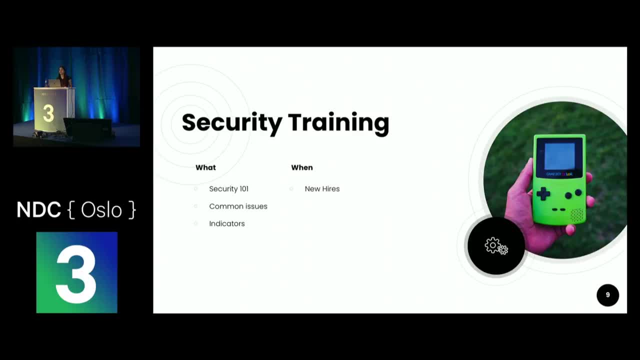 the company. you want to tell them early maybe some of the issues that have already been happening so that they don't repeat the same ones. So if there are certain vulnerabilities that keep coming up at your company or that you know is legacy code, you can let them. 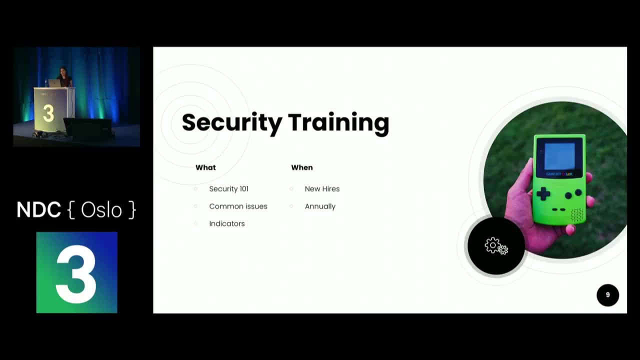 know, so that they're not doing the same issues Also annually. So this isn't something that should just be done once as a checkbox. It's over. It's something that's continuous because new things are coming out every year. So why? As I mentioned, it's a scalability issue, But it's also really good for knowledge. 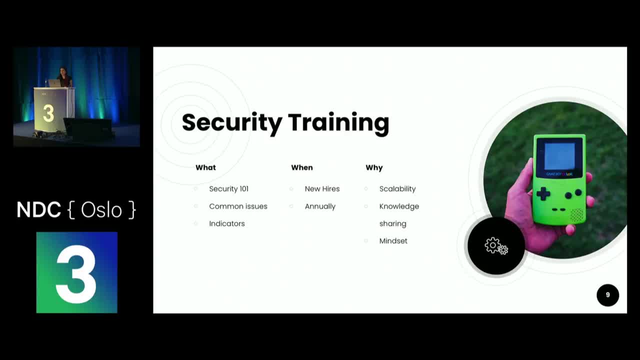 sharing. I mean, it's a really fun topic and a lot of people want to know more about it. So the other great thing is that it changes the mindset, so that it's not just: oh okay, security is something that's tech debt, We can deal with it later. It's something that. 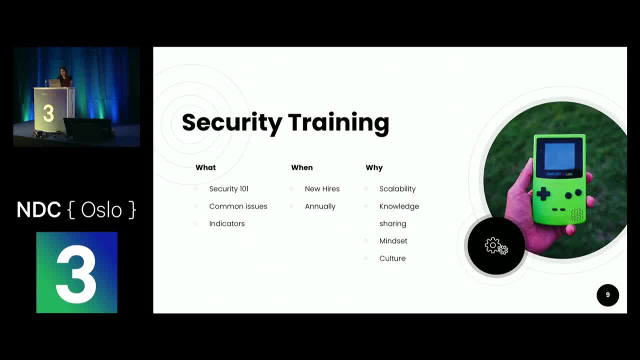 should be addressed as it comes up, And it also changes the culture a little bit. So it's kind of giving someone a contact to reach out to if there is an issue And it needs to be something that's addressed immediately, At least you know who to reach out to, as opposed. 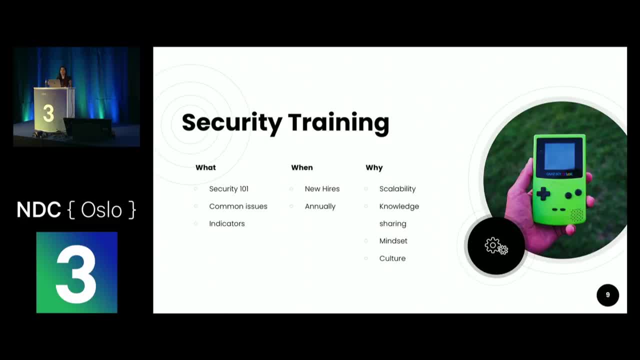 to maybe reaching out to the wrong email alias. It gets lost somewhere and never addressed. So an example of what happens if you don't do security training. A lot of you have probably heard of what phishing is, So this is one of those low-hanging fruit type things where 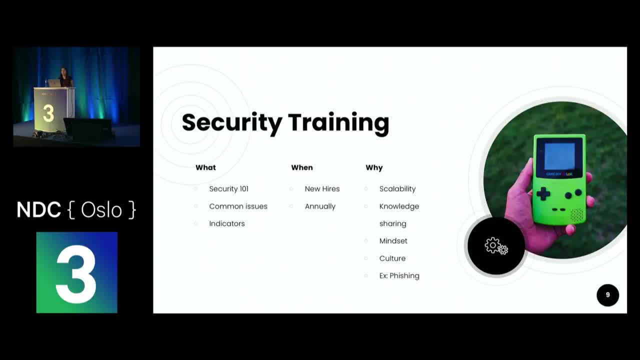 if someone wants to get through to your company, they can easily just send you an email and say, from your CFO to your CEO that says: hey, I need these numbers, I need them immediately. And you can spoof everything. You can spoof the headers, the email address that's coming. 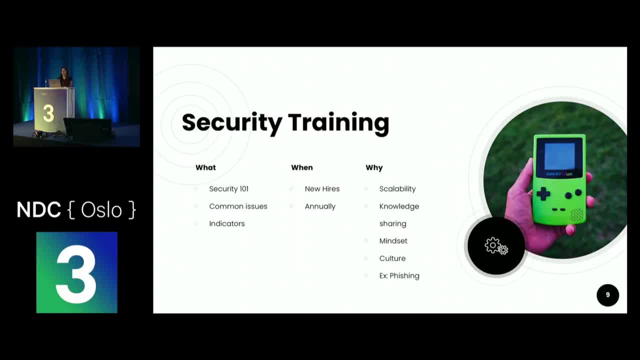 from all of it. But if you have training for your employees that basically says, hey, you should look out for these things and this is what you can check to make sure it's legitimate, then you're less likely to be attacked this way and to actually have it go through. 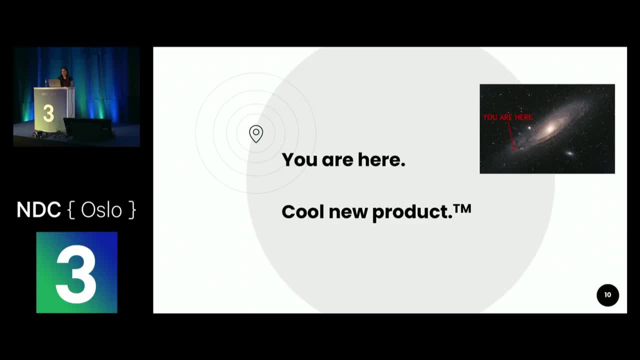 Okay. So on the timeline, you are here, You have this cool new product, trademarked of course, that you just came up with the idea for, and you want to begin. You're like, oh my God, it's going to be this amazing feature, It's going to change the entire universe and 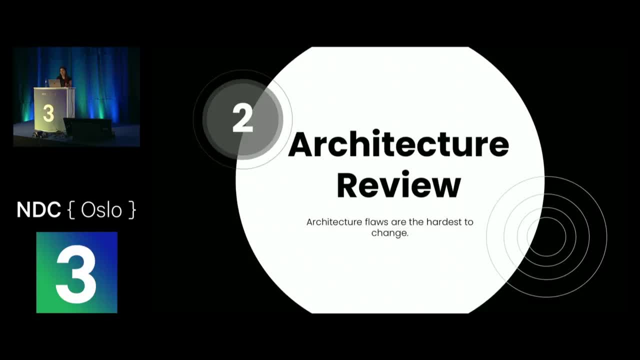 we can't wait to work on it. So where do you start with security? So you're going to start with an architecture review And you want to start here as early as possible, just because these are the flaws that are really hardest to change later on. It's not something that. 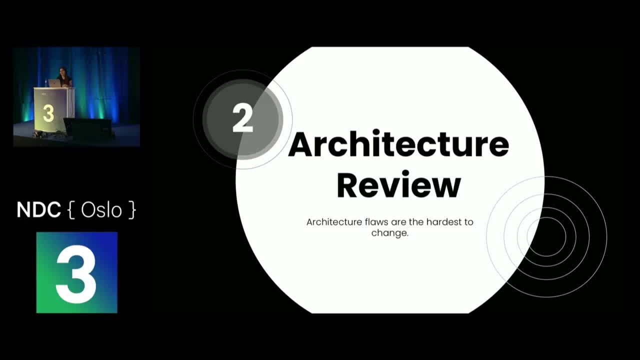 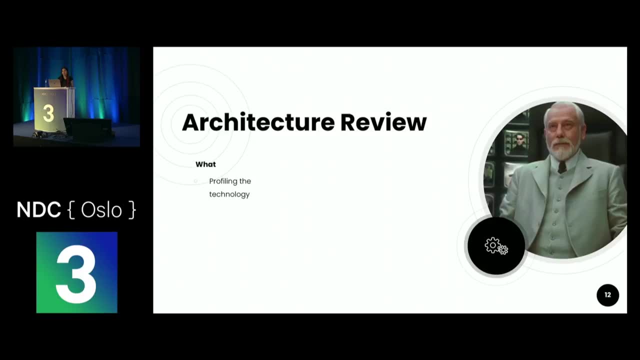 you can easily just ship out, Ship a hot fix out for and be done with. It's something that involves sometimes years' worth of work. So an architecture review, What it is is really profiling your technology, Seeing what specific things you're using- maybe AWS, Lambda, anything new that's coming out- Analyzing 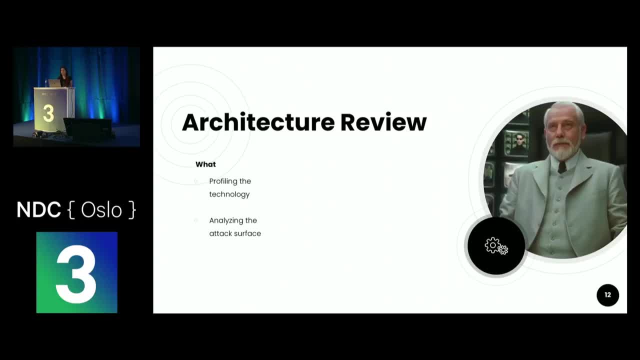 your attack surface. So, based on what you're specifically using, how can people basically attack that? And it's also ensuring it's not vulnerable by design. So there are so many products out there. I'm sure if you've seen the other security talks where a product was built with all these- 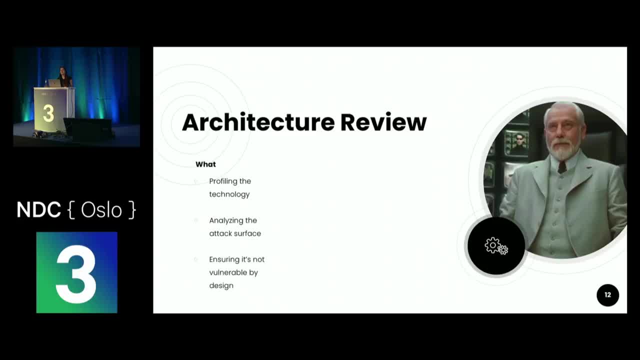 huge flaws in it and they rely on that. And the problem with that is that you have to come up with an entirely new product just to fix what was wrong in the first place. So when you would do it is product planning as soon as possible really, And why you would. 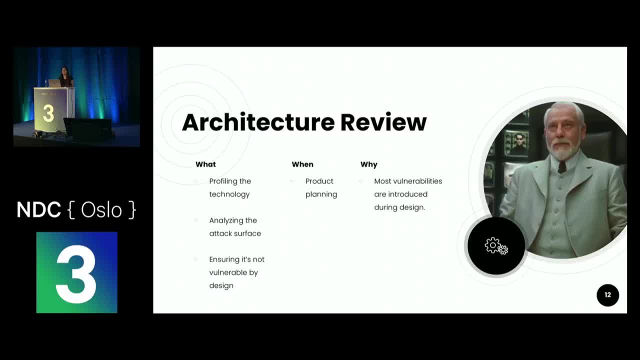 do? it is that a lot of vulnerabilities are introduced during the design phase. Like I mentioned before, they really are the hardest to change And this way you can be secure by default, which is basically making sure that all of your default presets are also secure, so that you're not going in later and telling your 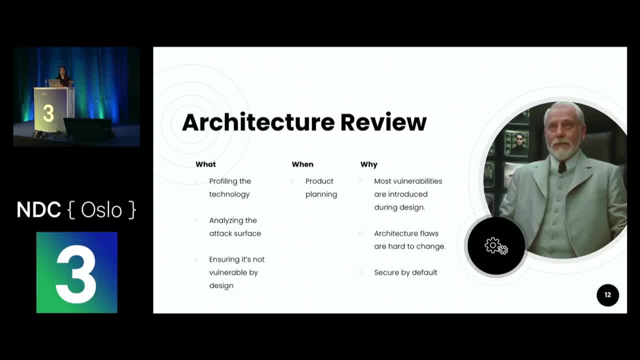 users. hey, if you want to be more secure, you can turn on this feature. It's better to be secure by default, because then if a user wants to use an insecure configuration, they can basically have like a pop-up that says: okay, you are being insecure by doing. 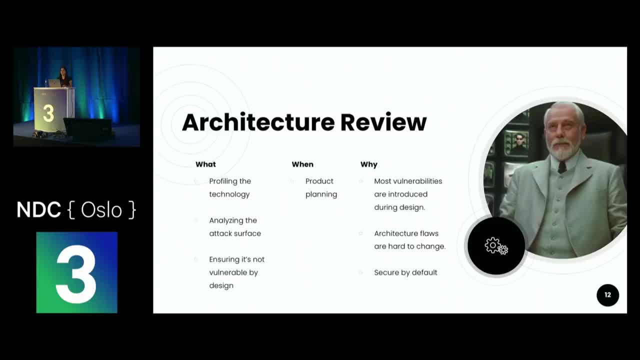 this. The responsibility is now on you and not on the company developers, anything like that. And this is the architect from the matrix, in case anyone needs the reference. So the architecture review is to make sure that you avoid things like this Where you. 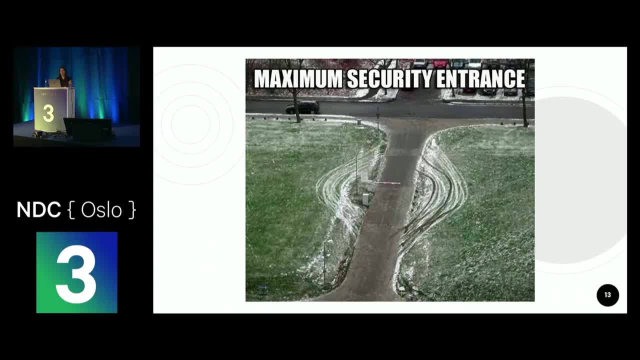 have the best intentions you're like. you know we'll put a security gate, It's going to be all fixed, We'll have a really secure product, But you don't think about the other ways that people can get around it, even though it might be obvious later on. 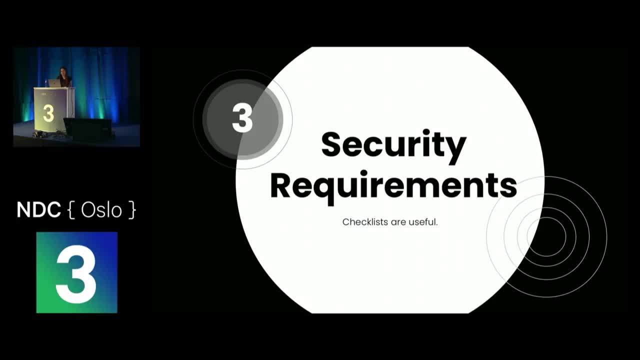 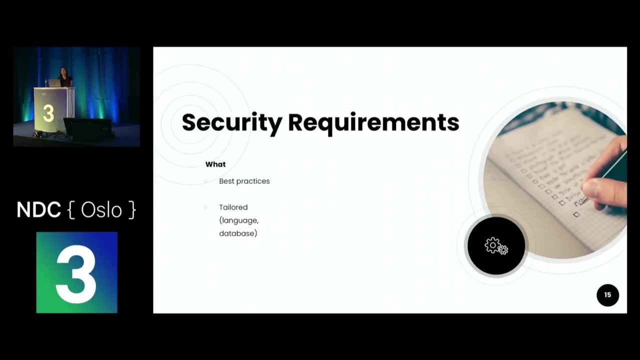 Okay, So that leads me to security requirements, And this is mostly a checklist. I'm going to show you how to do that. So it's really the best practices and it's tailored very specifically to the language and the database and all other specifics that you're creating. 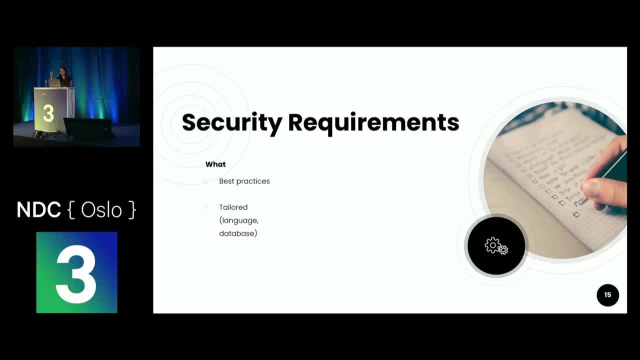 So it will have like a questionnaire that says: okay, if you're using this, this, this, these are the main requirements that you should be thinking about early on as you're building it. So you would think about it once you have confirmed architecture, once you know what. 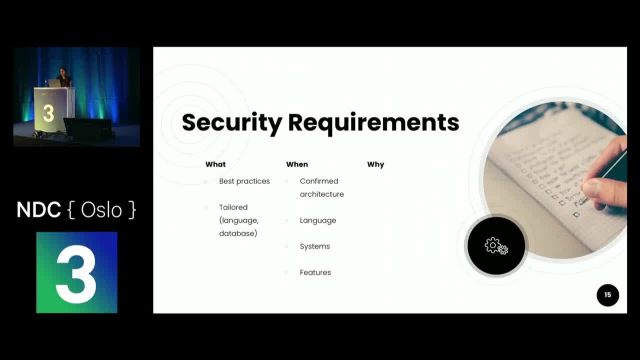 languages you're using, what systems features, things like that, And it's a great checklist, But the amazing thing about checklists is that they can easily be translated into tickets, which you can then add to your sprints that you can complete while you're building, as 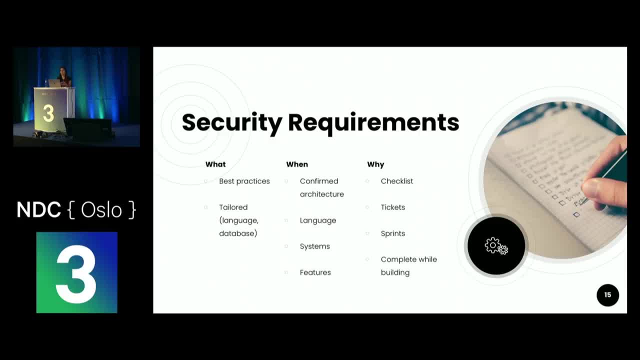 opposed to trying to add some security items onto your sprints later on when everyone is just super busy. You know you've got all these crazy deadlines and you're trying to bolt something on last minute. So and some tools for this. One of the tools is SD elements. They will definitely translate. 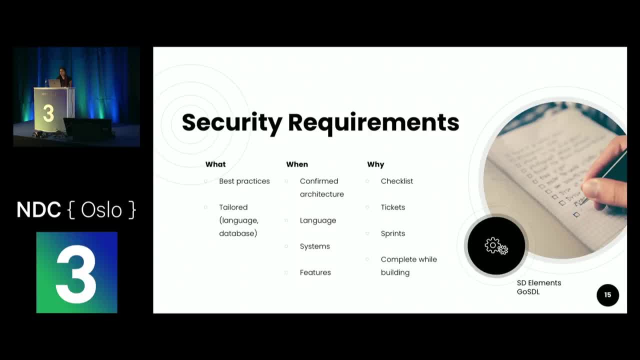 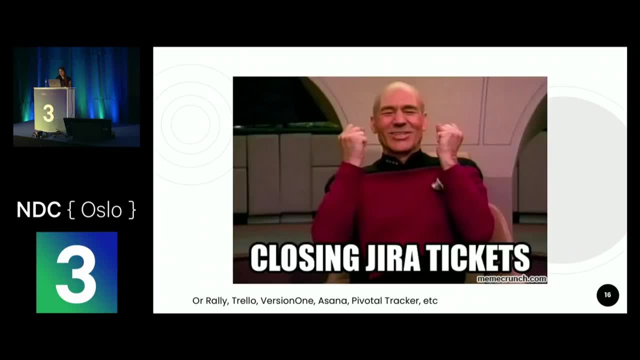 things directly to tickets, And one that came out just recently is GoSDL. It's by Slack and I think they just open sourced it a couple months ago, So I don't know about you guys, but I love closing JIRA tickets or Rally Trello version. 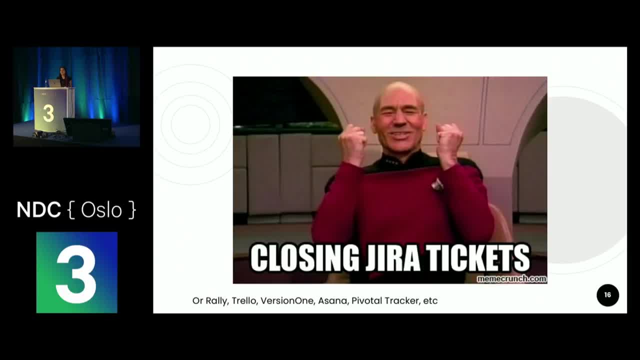 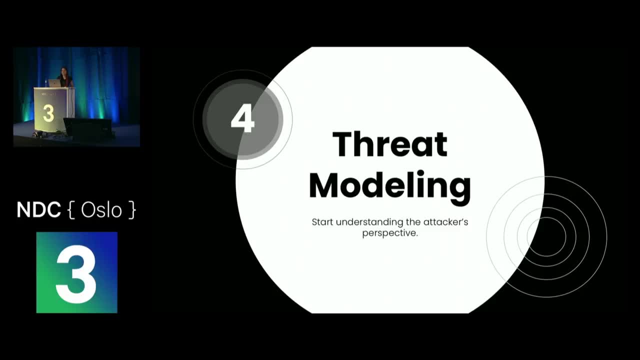 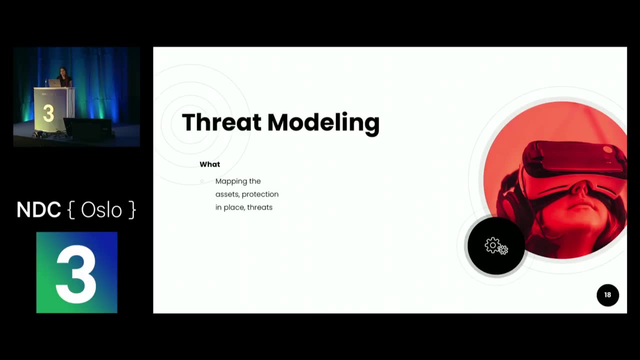 1, Asana, whatever you guys use, I like ticking things off. It makes me feel a lot more accomplished with things, So it's always good. So threat modeling: This is starting to understand the attacker perspective. Okay, So it's really mapping your assets, all the different individual things you're using that. 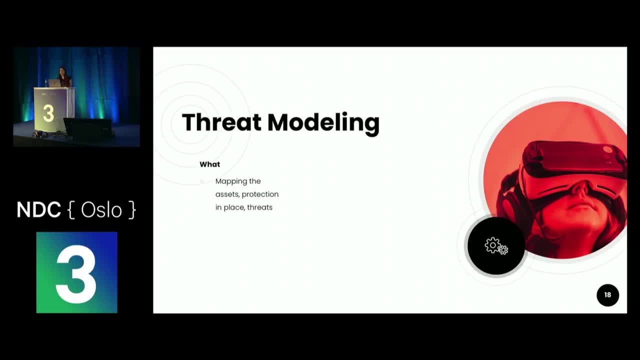 you might want to protect the protections that you have in place for those assets currently and the different threats that would try and attack that. So it's really understanding your threat vectors and I'll show you why in an example shortly. So once again, you do it once you have the confirmed architecture, preferably when there. 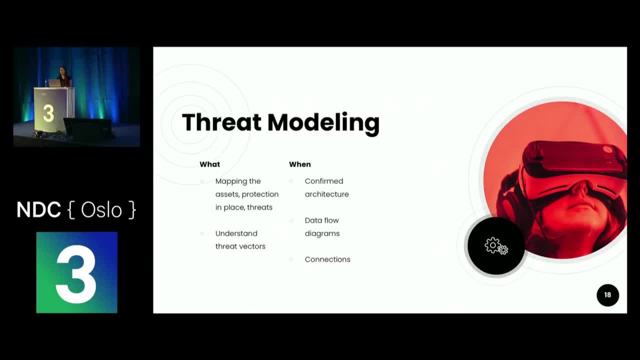 are data flow diagrams, because then you understand the connections more And some areas of the application that you might want to start drilling down into. So this will definitely help you lock down the easy attack paths. It's also a really nice visual for looking at later on, like, say, a couple years down the line, when someone 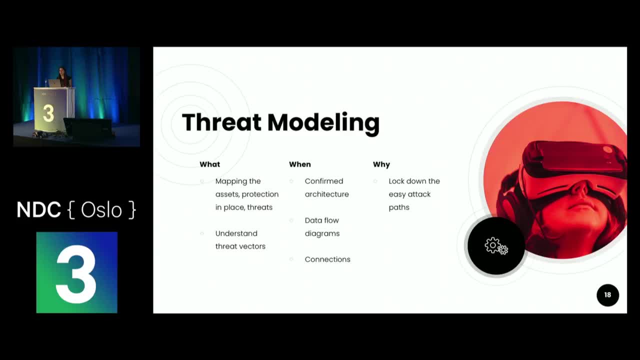 is like: okay, how does the application work and how are we trying to? ‑‑, how has it been secured previously and what are the new features that we're bolting on that might change this? Okay, Okay, And some of the tools are the Microsoft threat modeling tool and the OWASP threat dragon. 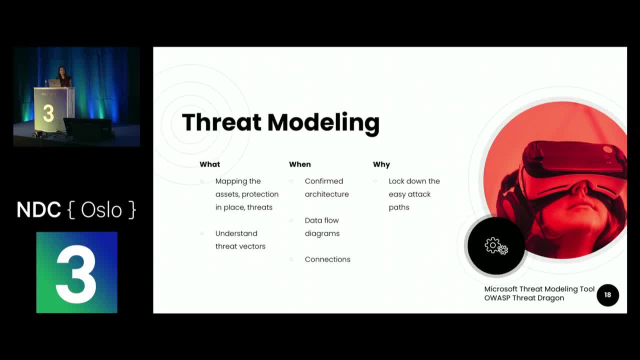 But honestly, right now I do this more manually, because a lot of these tools will give you a huge, huge list of results that you kind of have to filter through, and it's actually faster to just look at it yourself. So that's my two cents. If you absolutely love the tools, go for it. 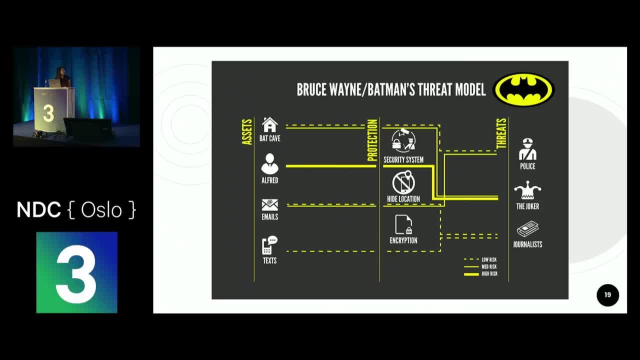 Okay, So an example of a threat model. So you've got your assets on the side here, Say: it's Batman, You've got the Batcave, You've got Alfred. of course, Emails, text messages, things like that. 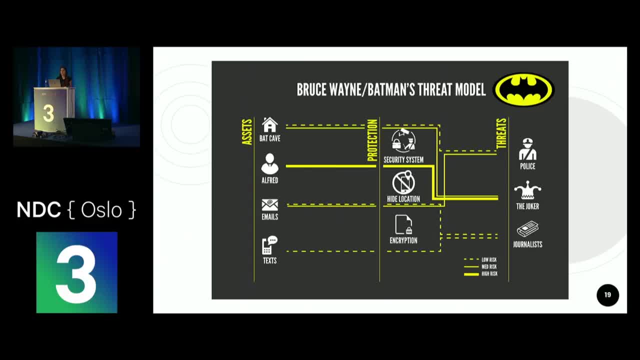 And what you have in place to protect these assets is security systems, the hidden, secret layer and some encryption, And the threats that Batman has is the police, mostly the Joker, and journalists, of course. So when you're looking at a threat model, you want to map everything out, starting from 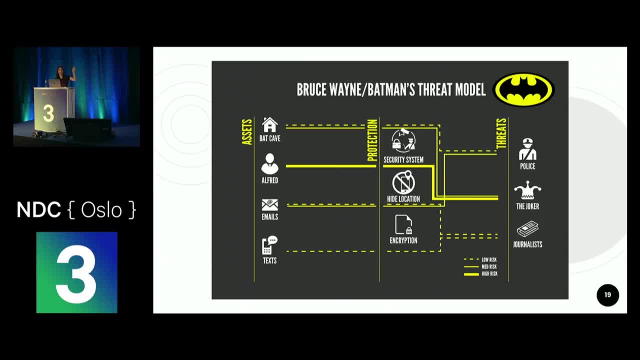 assets to threats, but when you're looking at the threat vectors, you go backwards. So you look at the threats and you say, okay, of the threats, which one is going to be the most likely to be attacking me? And it's probably the Joker, because he seems to have a penchant for Batman. 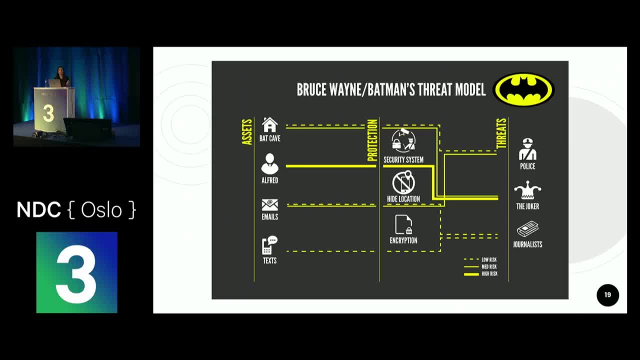 And he's probably going to attack via the security system, because he's more of a smash and grab type of villain And one of the things that he would try to get to is Alfred, because, of course, Batman really cares about all the people around him, so that might be a weak link. 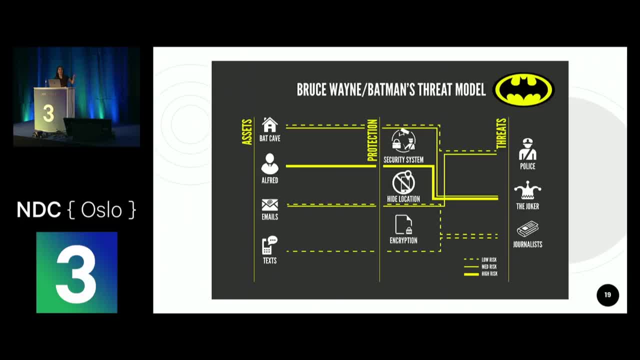 So that's basically how you would map the areas that you want to make sure you lock down the most, because you're looking at your assets and you're saying, okay, of all the assets, which ones are most important and which ones can be attacked via the threats. 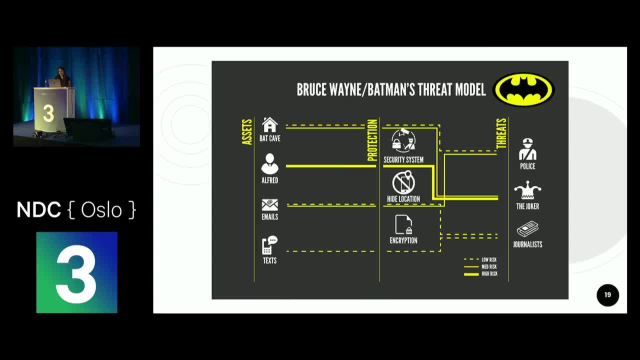 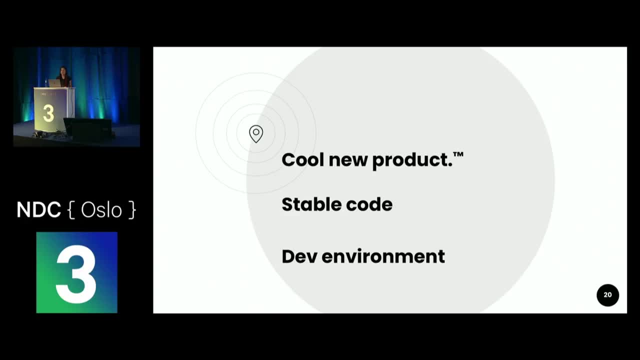 and how to lock that down, everything in between. Okay, so back to our timeline. We've got this cool new product again trademarked, of course, And you have stable code now and it's in a dev environment. So what do you start doing? 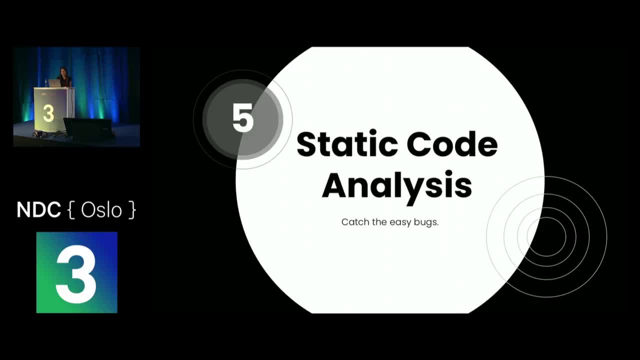 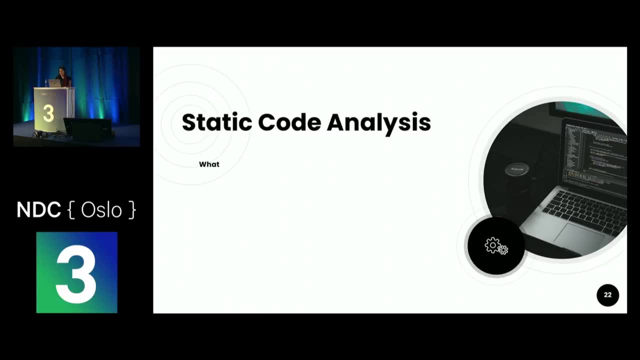 now. So there's something called static code analysis and this is basically catching some of the easy bugs early on. Okay, And what it is is really scanning your code for obvious issues. So it'll go through everything and say: your feature is a new search field for your product and you're taking all this. 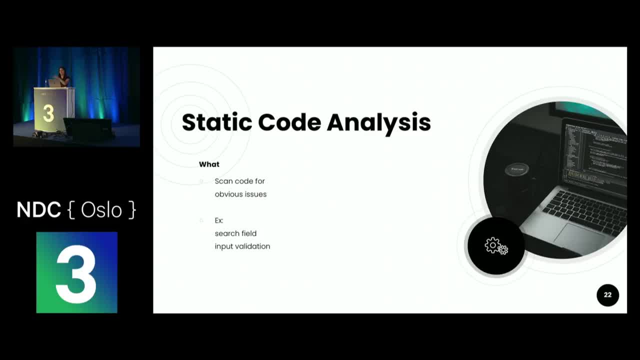 user input but you're not doing any input validation. You're just throwing it straight back and then fetching it again. That is something that would come up in this and basically have a red flag and say, okay, for this specific line of code you're not doing input validation. 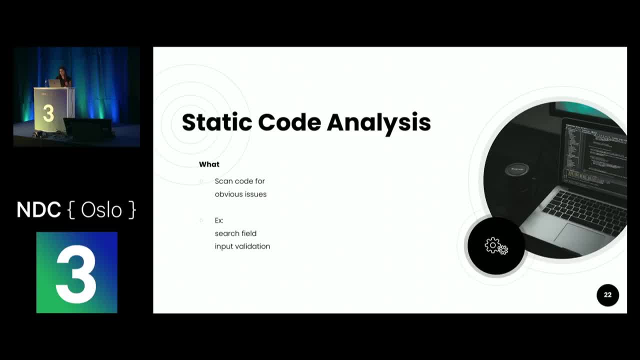 These are some of the things that you could do and some code snippets that you can add into it. So you would do this as soon as the code is checked in, preferably as soon as possible, because it's a lot more difficult to go back later on and find exactly what you were doing. 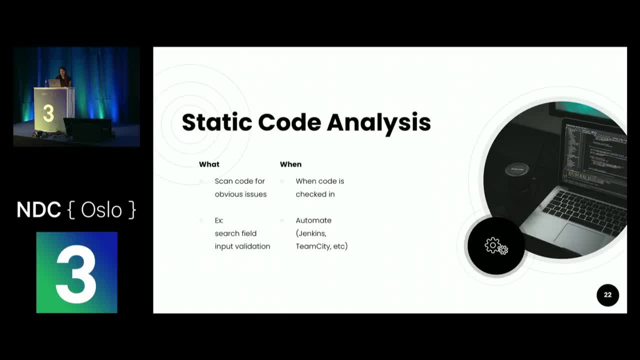 with that specific area and bolt it on. It's also something that you can easily automate either in Jenkins, TeamCity, whichever one you're using, And essentially it's catching all the issues as soon as the code is available and remediating. 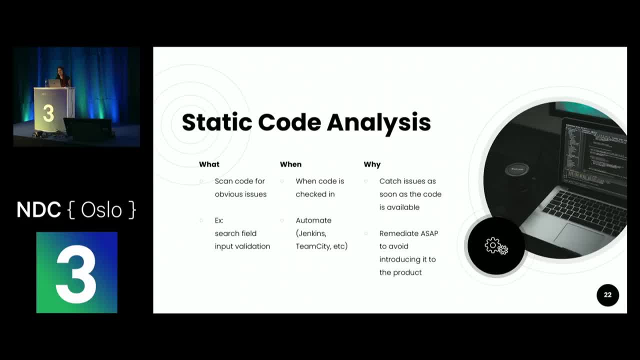 it as soon as possible, So that you're not introducing it. You're introducing it to the new product, And one of the main reasons why you want to do this as soon as possible as opposed to later on. once the product is all released and everything is that, you'll have a lot. 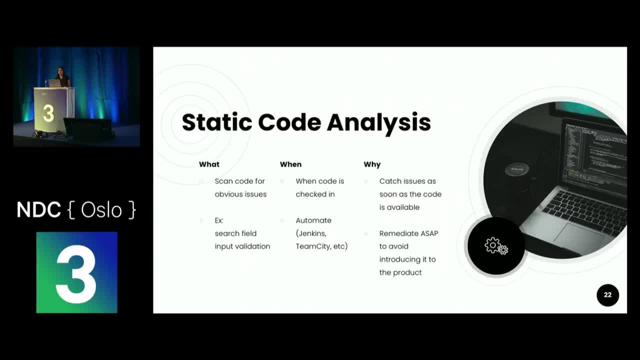 less results coming up and a lot less things that you need to filter through, And you can start cutting things off at the root as opposed to trying to fix all these different areas. And some tools for this- Veracode Checkmarks Fortify. they all basically do the same things. 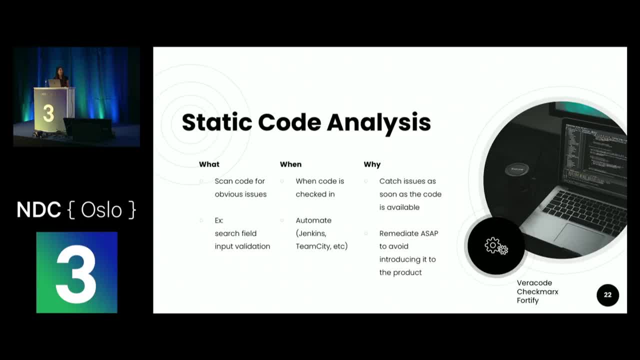 What you want to be careful with When you're choosing a tool is if they support certain languages. So there's no one tool that will support absolutely everything out there. So you really want to take a look at what you have specifically and make sure that it's. 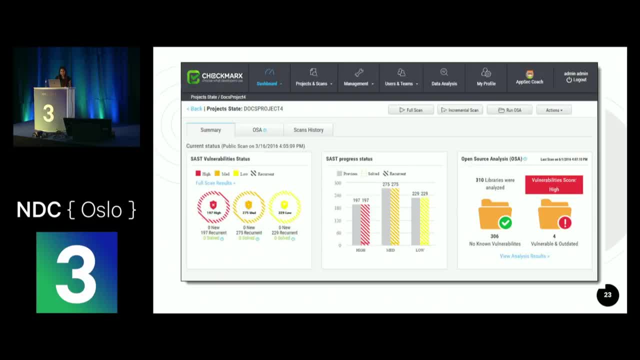 all going to work with the tool. Okay, So this is Checkmarks. It's one of the stack analysis tools, So just to give you an idea of what it is- And full disclaimer, this is a snapshot from online. None of this is internal to anything that I've worked on. 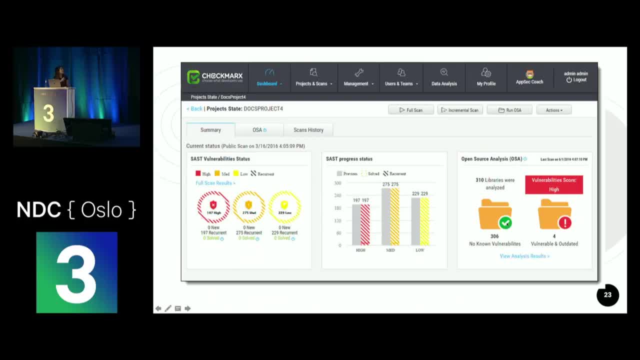 But you can see on the bottom corner here that there are 197 highs and they're all recurrent, And the great thing about automating these scans is that it will tell you from the last scan to this scan, have there been any new vulnerabilities that someone has introduced? 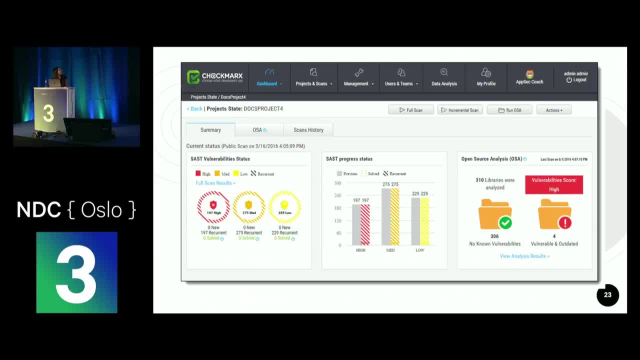 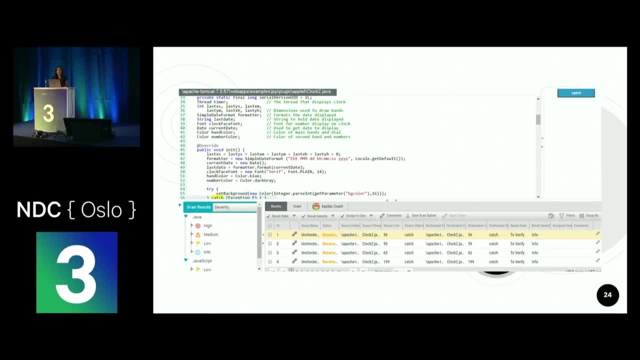 to the code. The other great thing is that you can drill down and see the exact line of code that is causing the issue And fix it there. One of the other great features is that you can start seeing which ones have already been fixed and need to be verified via another scan. 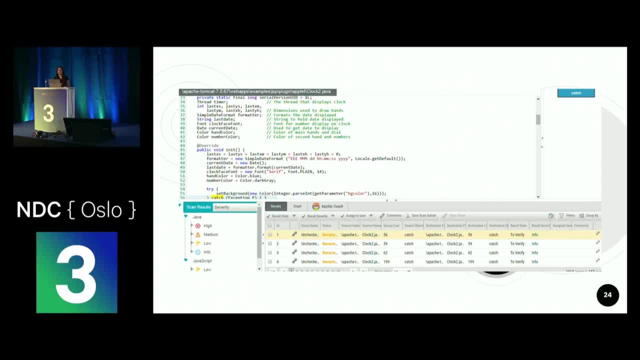 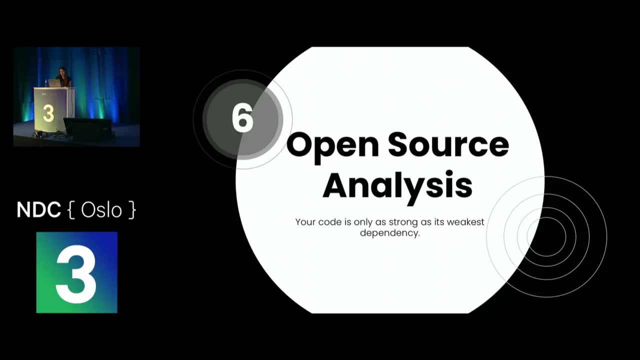 Or which ones are false positives, and they'll just not show up anymore. So it's just an idea of what static code analysis would look like. So, open source analysis, Your code is only as strong as its weakest link, And I say this again: 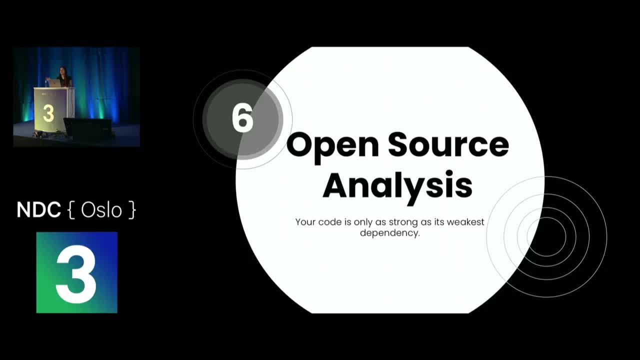 You could write the most perfect code, Perfect, secure code possible. It could be pristine. You're so proud of it. But it doesn't matter if you add an extremely weak dependency to it, Because then you're introducing this huge vulnerability to your code base and to your 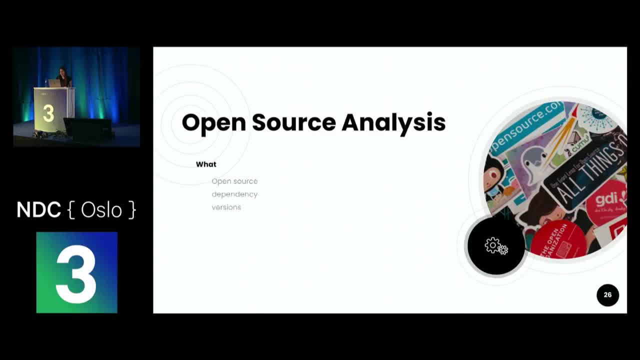 product. So what open source analysis would do is go through all of your code and pull out the dependencies and the specific versions that you're using. This is really useful because sometimes we forget which version we're using. Sometimes we wrote something years ago. 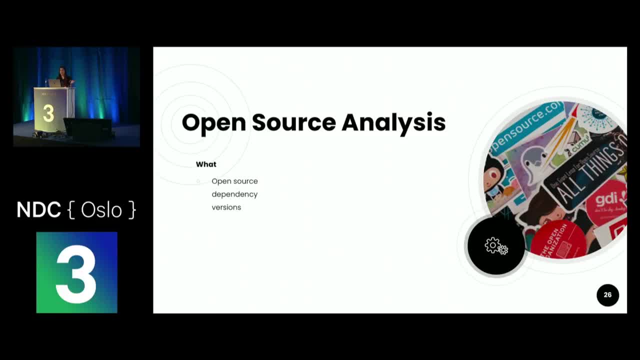 And we just never thought about it ever again. This will pull all of those up and bring it to the forefront, And it'll also tell you the known safe versions. So in some cases, if it's something you haven't worked on in a really long time, it might. 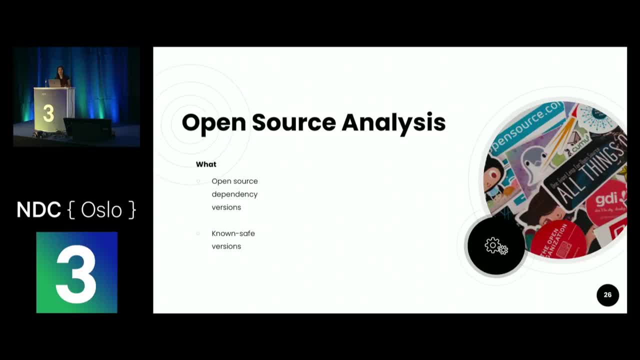 be a major update that you have to do, But in more likely scenarios, it's usually just a couple versions that you have to change. So this is something that you would also do when code is checked in, And you would automate it again with Jenkins and TeamCity. 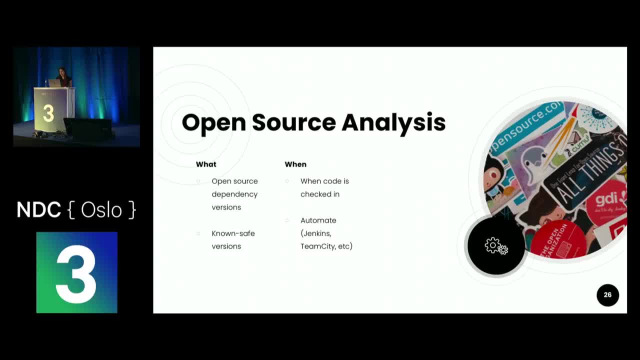 So that it just runs automatically. It runs on its own and you don't have to think about it. So why are we doing this? As I mentioned, you don't want to introduce critical vulnerabilities And everyone's kind of like: yeah, obviously, of course you don't want to do that. 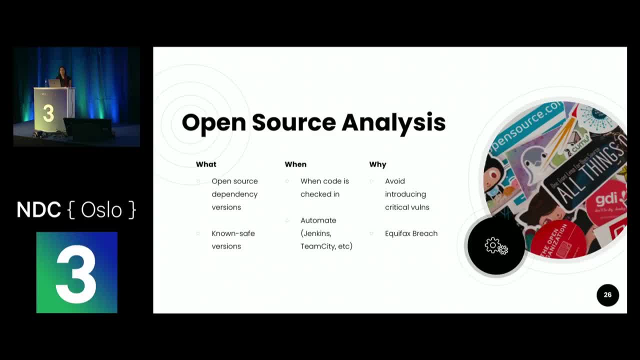 But I don't know if you've heard of the Equifax breach. So Equifax is this huge credit reporting agency in the US And they basically deal with a lot of really sensitive information like social security numbers- I believe it's called personal identification numbers here. Credit card numbers, date of birth, a lot of information about you- And they had a breach where 146 million users were affected And just to put that into a little more perspective, that's half the population. So every other person in the entire United States had their social security numbers taken. 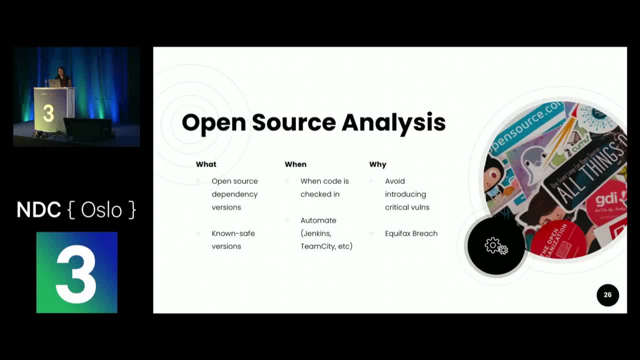 within this breach And the thing about this is that it was a really easy attack. It was an Apache Struts vulnerability that they could have found and fixed by doing open source analysis and seeing that they have this critical issue within their product and within their infrastructure. 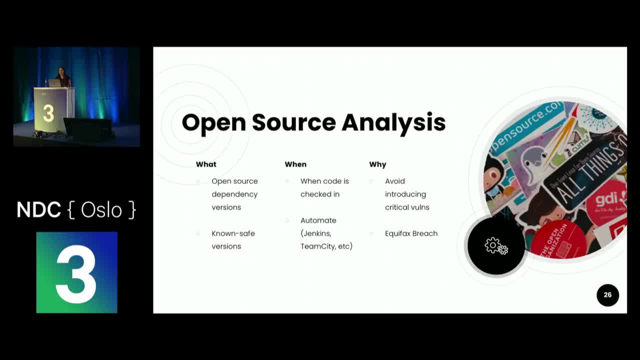 So I really can't emphasize enough how important this step is. If you don't do anything else, at least do this. It's something that you can set up super easily. There's a lot of open source versions out there that you can just throw into your code. 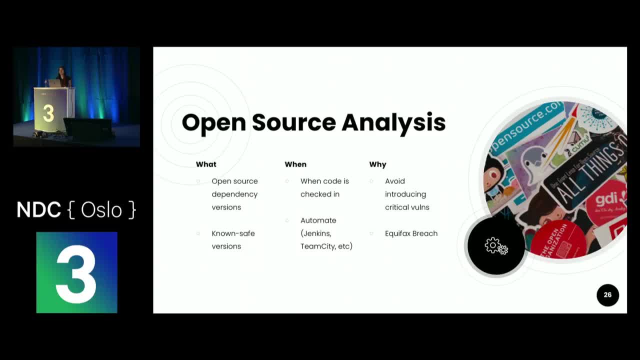 really quickly And it will light up like a Christmas tree with all the red things that might be in your code. There we go. So some tools that you can use for this: There's white source, source, clear and sneak- And there's actually a lot of tools that have open source analysis integrated into it. that 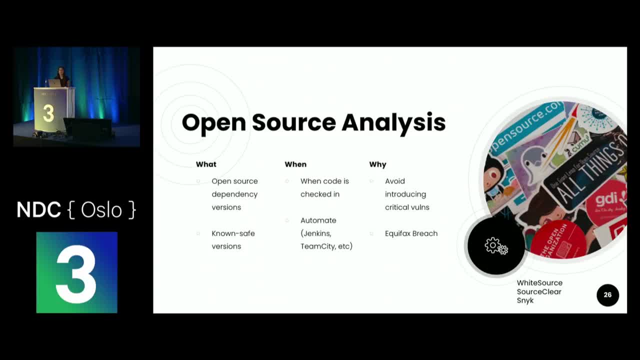 use these tools as their back end. So if you use check marks, you can add white source on top of that, so that it's all in one pane of glass, which is kind of nice, because when you're automating it's just one thing. 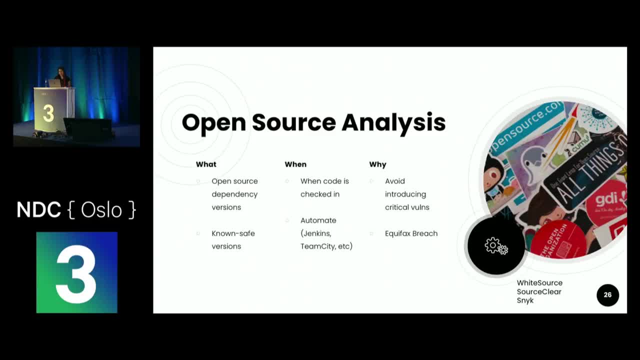 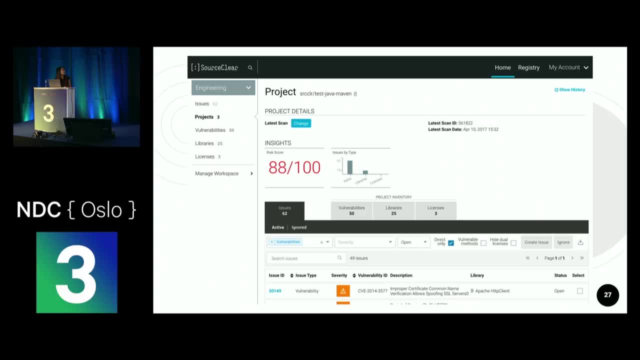 to do, as opposed to two separate ones. Okay, Great, Okay, So what does it look like? So, again, this is pulled from online, So it'll tell you generally what your risk source is, but, more importantly, on the bottom half of this screen, it'll tell you how many issues, the vulnerability, the actual CVE. 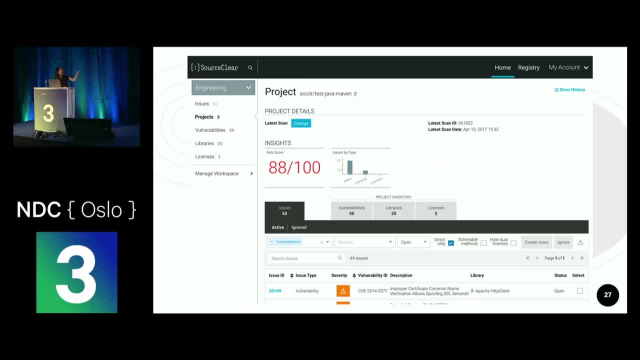 ID associated with it and what it is, And I couldn't find a screenshot of the further drilled down version. but if you click on that vulnerability, it will tell you the exact libraries that you're using or dependencies, things like that, And it'll actually give you the code snippet to just do a quick diff and change it all. 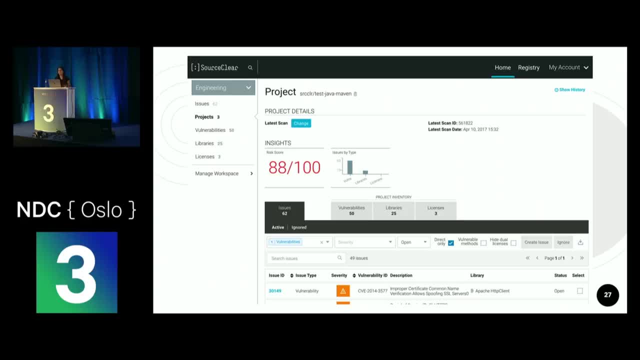 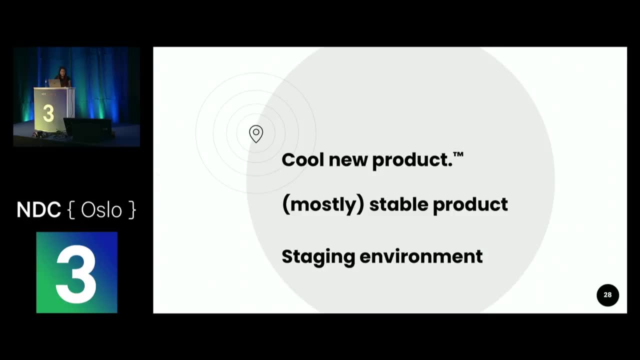 So, assuming it doesn't break anything, it's not a huge update. it's relatively easy to change over. Okay, So you've got this cool new product and it's now mostly stable. Hooray, And it's in the staging environment. 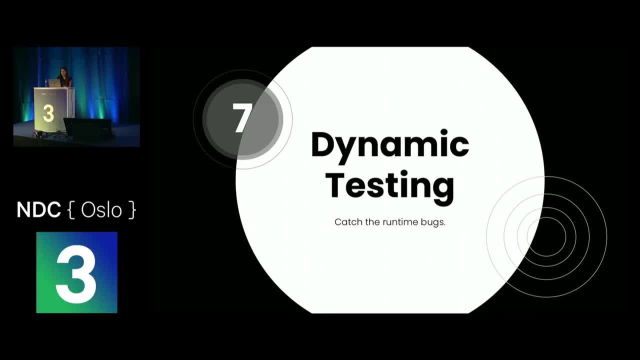 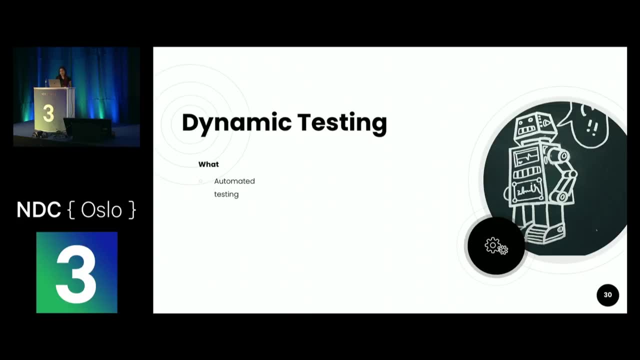 So what do we do now? So dynamic testing. This is catching your runtime bugs, as opposed to static, where it's just specifically the code. So it's automated testing and it's a black box approach. So, for those of you who don't know what a black box approach is, it's basically testing. 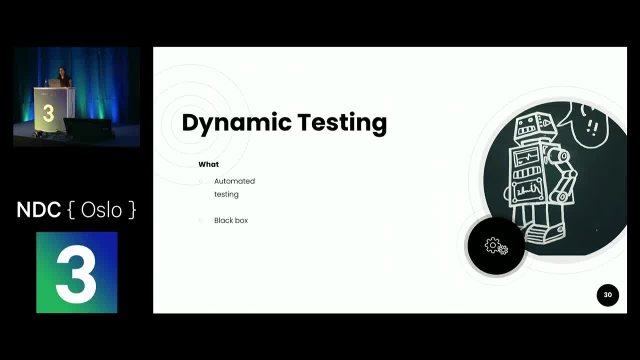 something with zero context of anything in the back. So they don't know about any of the code. They don't know anything about what the application does. It's just specifically trying to find the easy issues. So you'd run this once you have the stable product and the staging environment, and usually 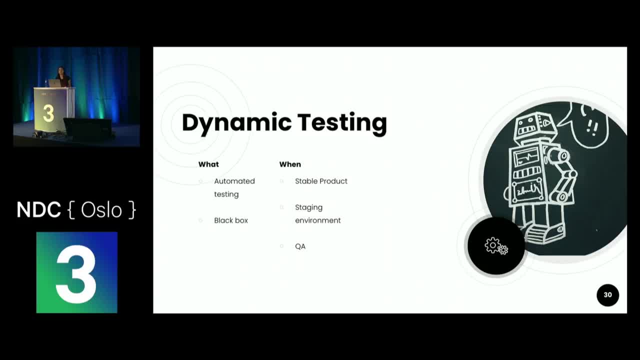 during QA itself. So if you're running any scans once your code is checked in, like using sonar cube or any of those tacking this on at the very end of it, would be best, Because then it's just automated, It's running on the back end. 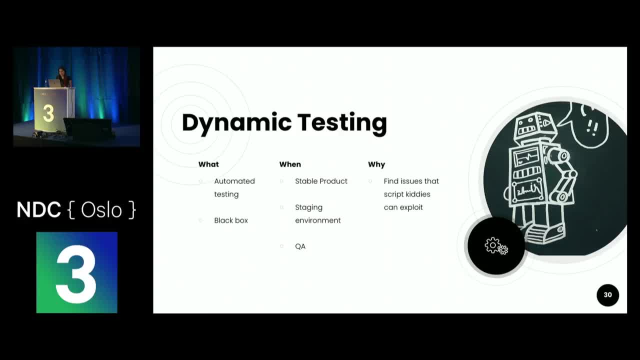 You don't have to think about it, So why bother? These are issues that script kiddies exploit more often than most, because these are kind of like the drive-by issues, So the ones where people are like, oh, why would anyone ever attack us? We're not this huge, huge company. Why would anyone take the time or even bother? And the answer is simple. Sometimes it's ridiculously easy where people aren't even targeting you. They might be targeting your customers, Or you might just be a jump box to get to someone else. 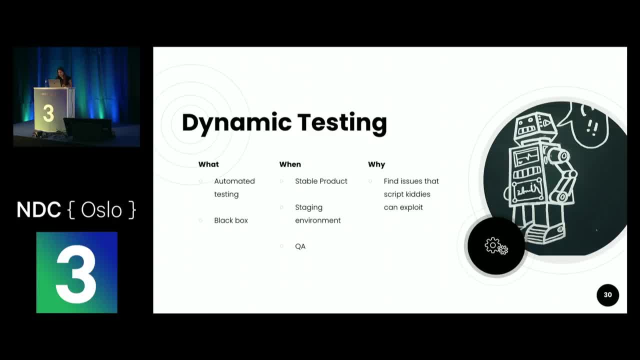 Oops, Sorry, There we go. Yes, Okay, And some tools. Easy. Some tools you can use for this are OWASP's app- This is open source- Burp and AppScan. So this is in order of price range. 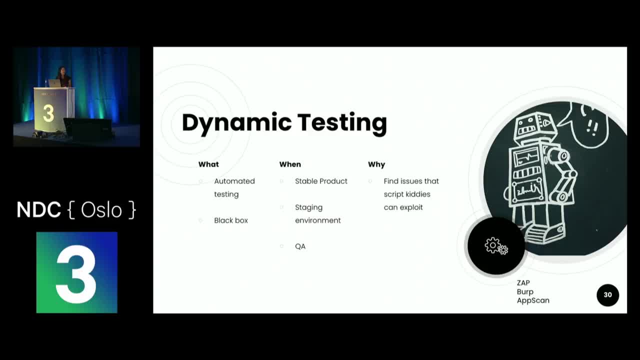 Zap is free, Burp is mostly free for the community edition- about $300 a year for the pro version, which isn't bad- And AppScan- I don't even know what the price is for that, because it's not something I'm. 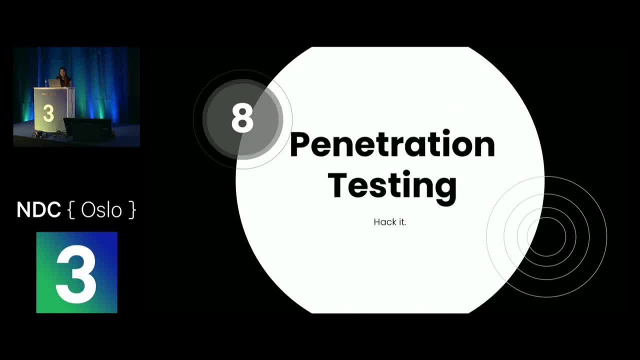 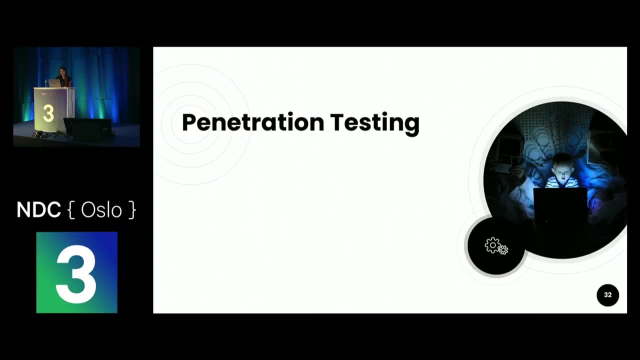 willing to fork over. So pen testing. This is my absolutely favorite part. This is the whole reason why I got into security In the first place, Because it's essentially hacking all the things. This is the fun part, But there's also a reason why it's at the very end, and I'll get into that in a second. 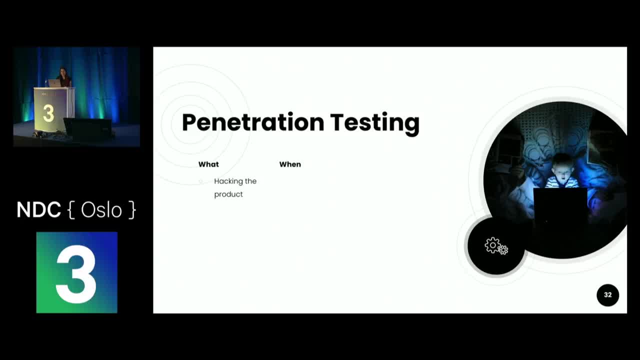 So pen testing, It's hacking your product basically like an attacker would- And you would do it definitely before your product is released publicly- Just because if you find these, if someone else finds these issues before you, it looks really bad in the media. 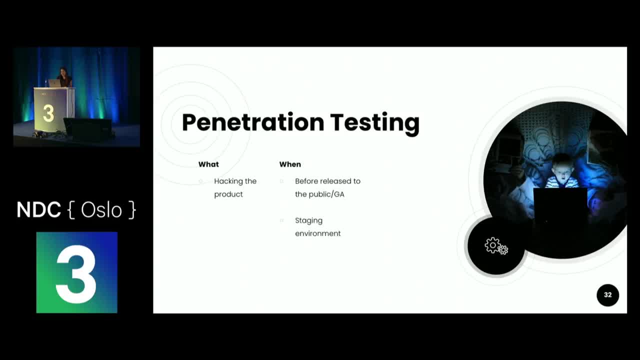 You get called out Not good. So you would do this again in the staging environment. but if you like to live dangerously, you could do it in prod. I don't suggest it, but you can do whatever you want, Okay, So why bother? 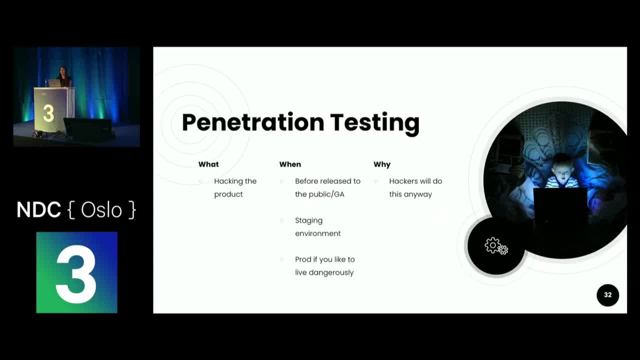 Hackers will do this anyway. Like I said, sometimes they just go for the low hanging fruit. You might not even really be a target. It was just really easy to do, And you might as well find the issues first and fix them before it's available to the. 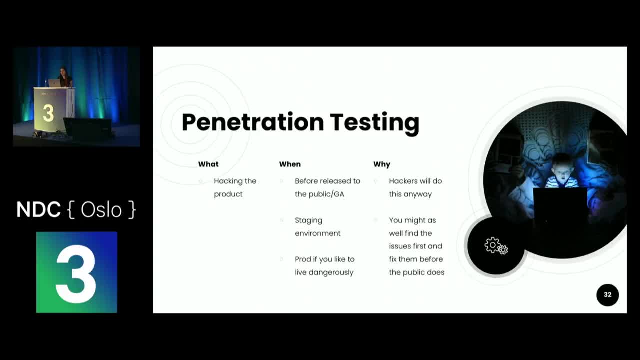 public. So one thing about this Stage is that if you've done everything else before this, you should not be having a lot of findings here. So you shouldn't be having like 20, 30 findings in a pen test report. 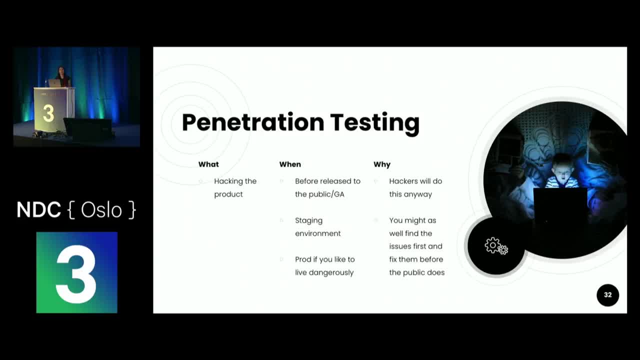 It should be really only the things that were difficult to find otherwise, So not in any of the other steps. And then some tools again for this: burp zap and app scan. They're proxies that can test your product And in general. 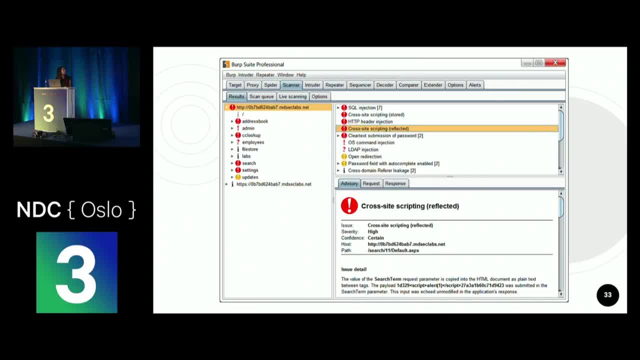 Okay. So an example of say what burp would look like. So this is just with a scanner. When you're doing an actual pen test, you'd start using all the other tabs, extensions, things like that, But just to give you an overview of what it might look like to an attacker if they're 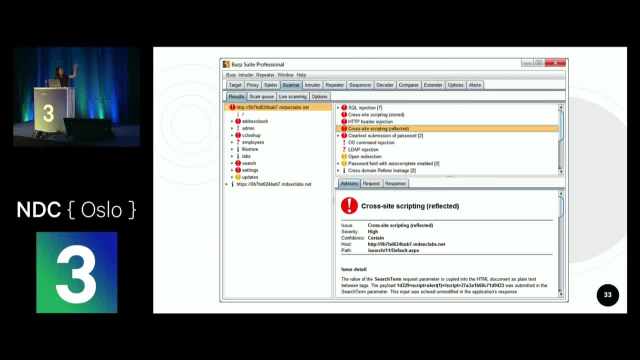 running an initial scan on your website, it'll pop up with all these different issues that are just immediate, So they don't even have to do anything at all to get to this screen. It's something that the tool will do for them. So when people are like: oh, how did you find that? 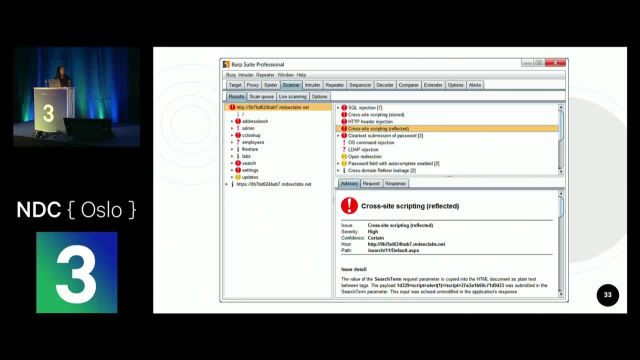 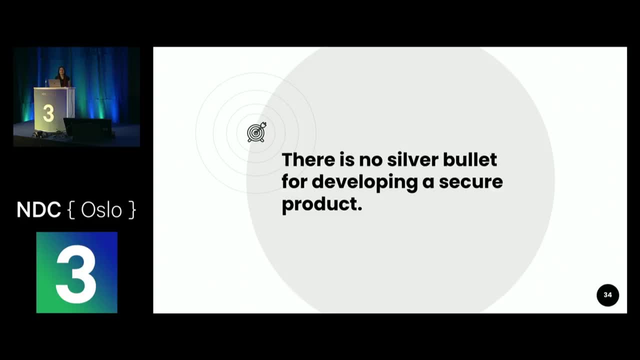 That's really hard, It's sometimes it's really not Okay. So there is no silver bullet to developing a secure product. I know it would have been nice if I could just give you an easy button and say, hey, just do this one thing and everything will be secure. 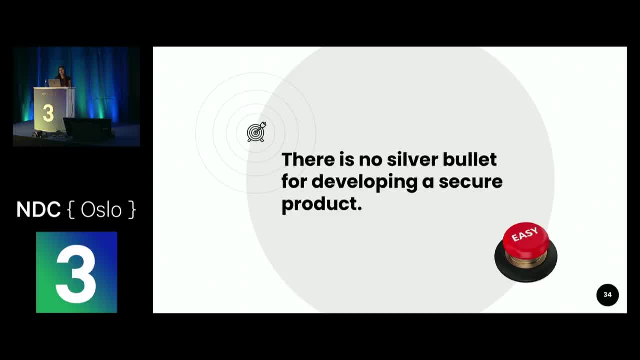 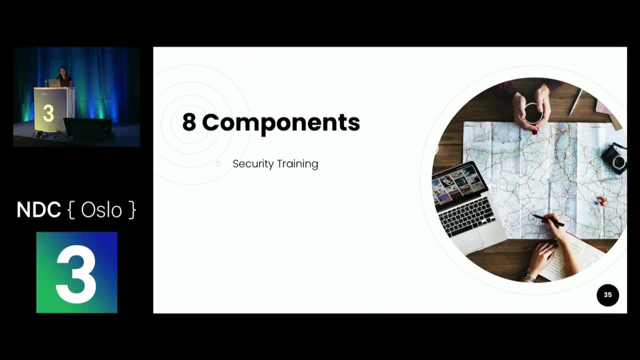 It'll all be perfectly fine, But that's just, it's not how it works And it's constantly evolving. So there were eight components that I went over: Security Threat, training, Architecture review, Security requirements, Threat modeling, Static code analysis. 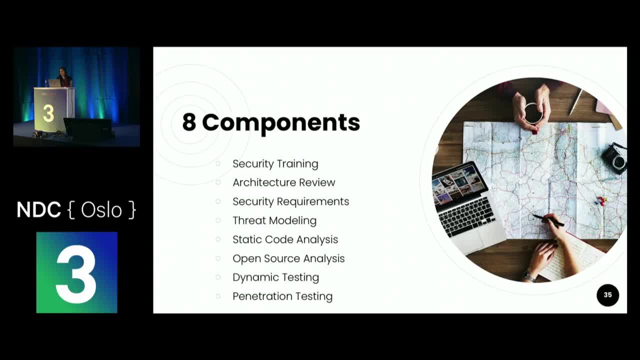 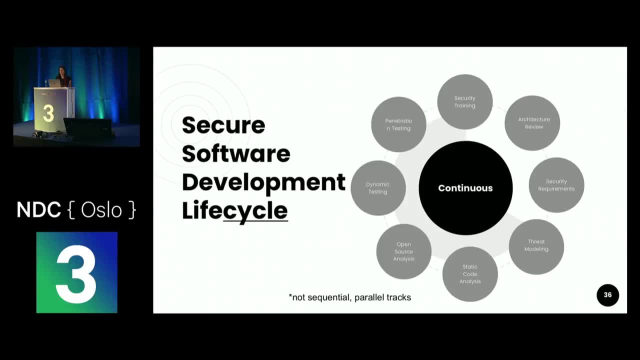 Open source analysis, Dynamic testing And pen testing. And the key thing to note about all of this is that it's not something that you iterate through once and you're done. It's actually a cycle, hence secure software development life cycle, It's continuous. 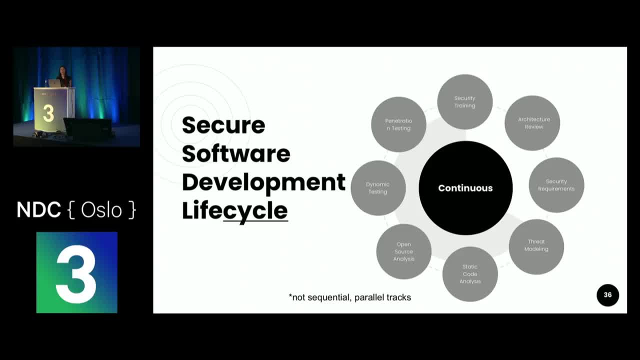 And along those lines. it's also not sequential. A lot of things are happening in parallel. So, for example, static code analysis And open source analysis- You'd probably kick off around the same time and they would both be running every time you check in code. 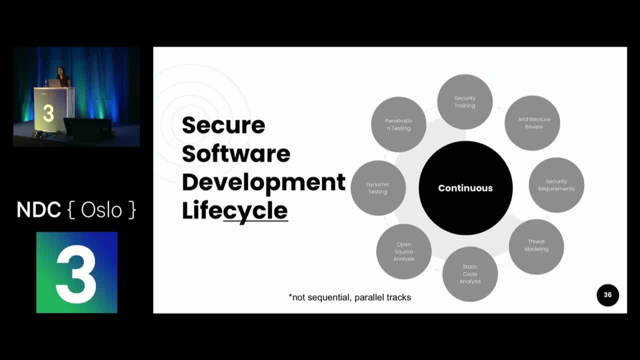 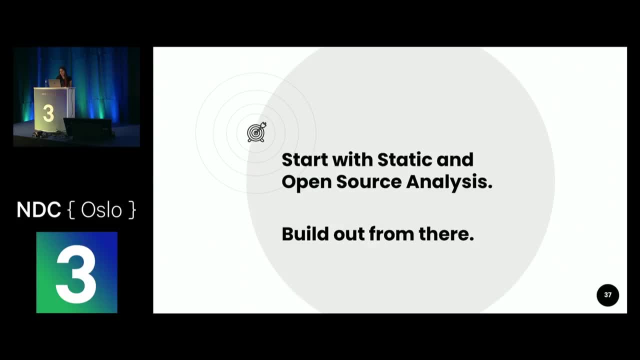 So it wouldn't be something that you just do once the product is entirely done. It's constantly happening, as development is constantly happening. Okay, So, coming to the end here, If you don't do anything at all, at least start with static code and open source analysis. 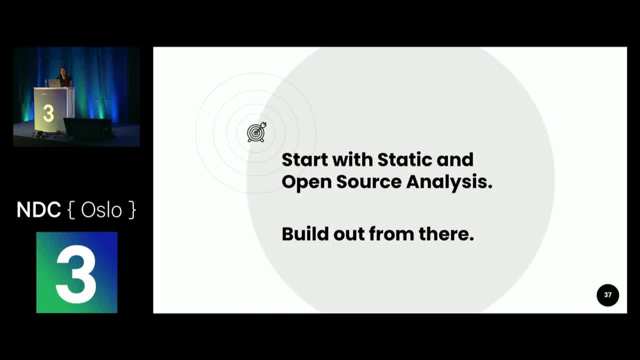 because this will give you the most bang for your buck immediately. If you start with pen testing, you might miss a lot of the other vectors, because the thing about pen testing is that it's usually a very narrow scope and it's usually a time box approach. 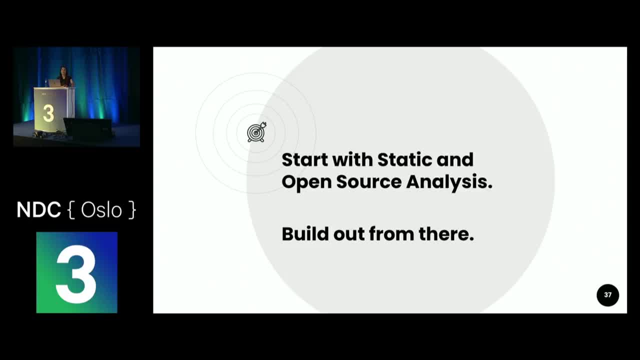 So you might find cross site scripting or SQL injection in a certain area of your application, but it might actually be prevalent in a whole bunch of different areas. You just didn't test for it in those. So if you do static code analysis it will at least pull out all the different areas. 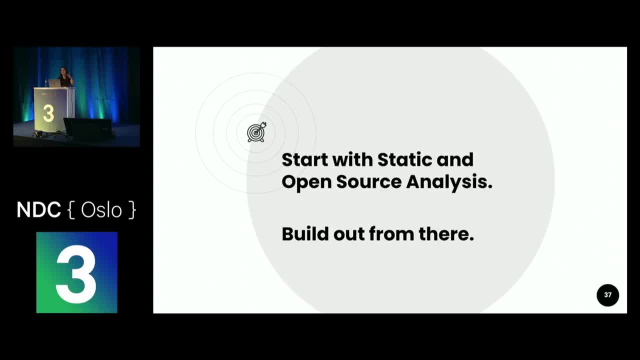 so that you can find a root cause that will fix all of those for you. Okay, So open source analysis fixes different areas, and then having to do it all over again, Open source analysis, just because these are things that a lot of people are hitting right. 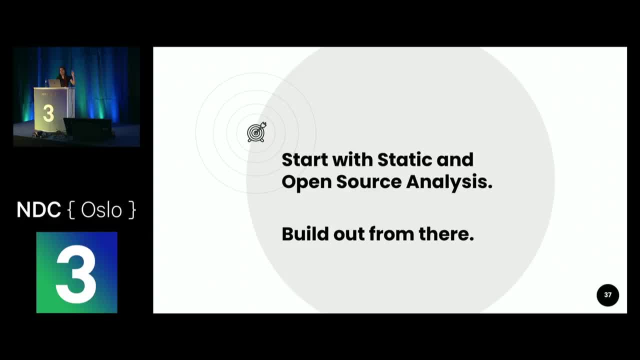 now, because it's really as easy as finding a stack trace that you're using a certain dependency and saying, like going to Google and saying, hey, what is an exploit for this? And then copying, pasting: That's it, Like it's really a no brainer. 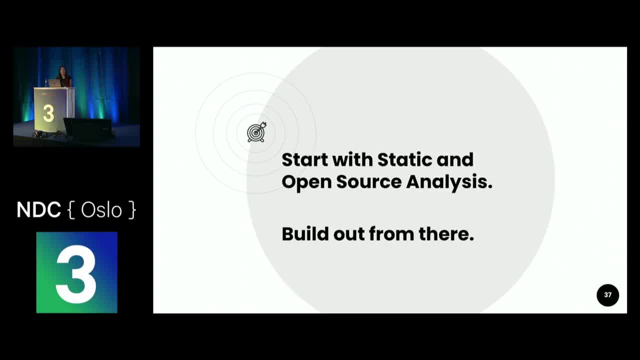 It's also really great to start with these because they're easy to automate, So it's less manual than a lot of the other steps within the process, And then you can kind of build out from there. So if you start with these two, then move to whichever ones else that are easier to. 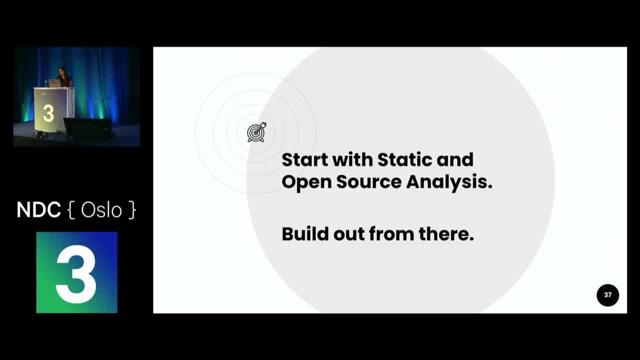 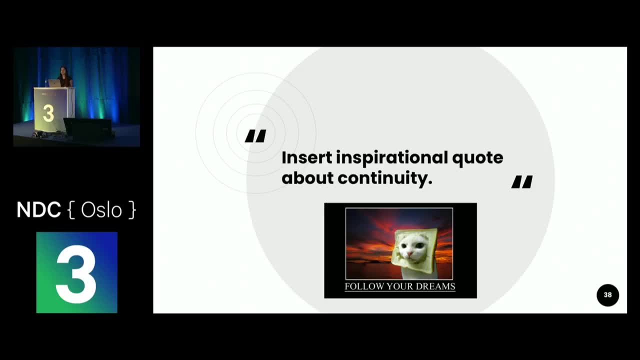 get to, then you'd be in pretty good shape. Okay, So with that, I leave you with this super inspirational quote about continuity, how life is continuous and development is continuous, and so is security, and a cat telling you to follow your dreams. 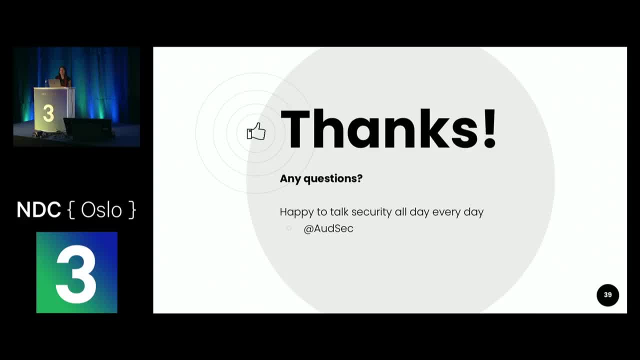 Thank you. If you guys have any questions, feel free to come up.